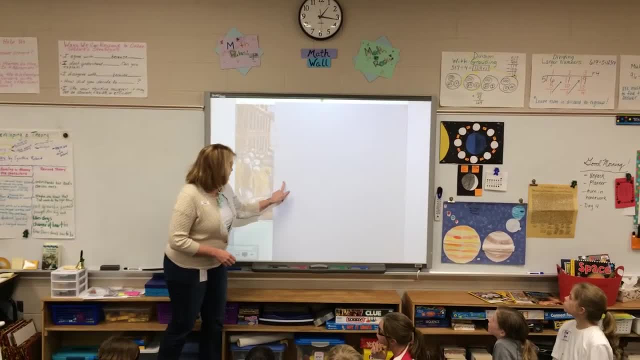 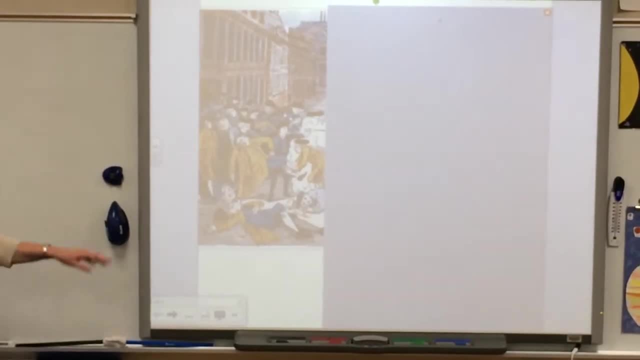 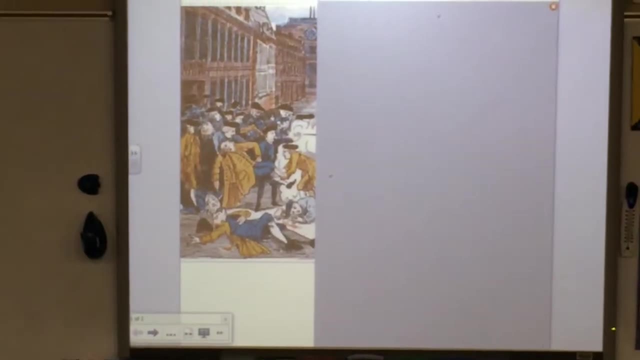 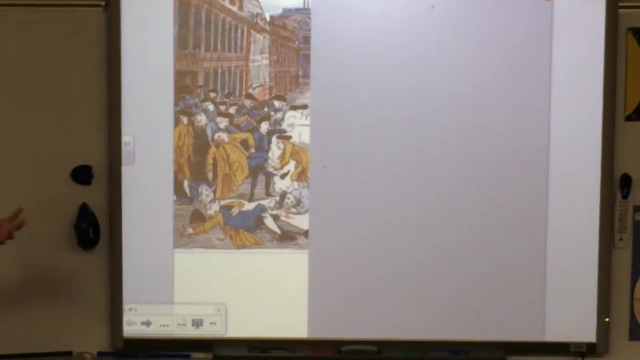 Ready. So this is all I want you to look at, And I want you to look at everything you see in this picture. You might know what. this picture is right Because it is very famous, And you studied Paul Revere last year, So just write down what you notice. 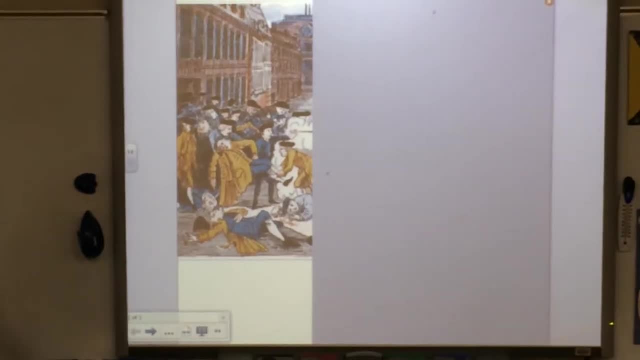 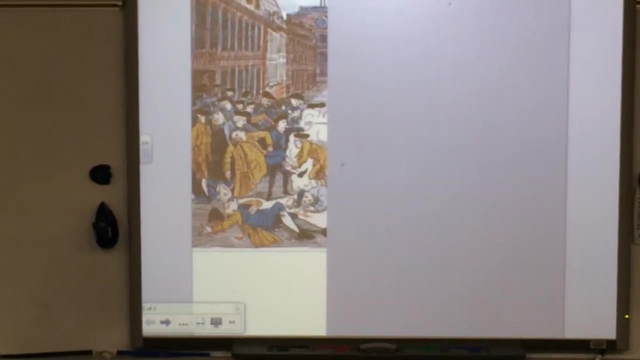 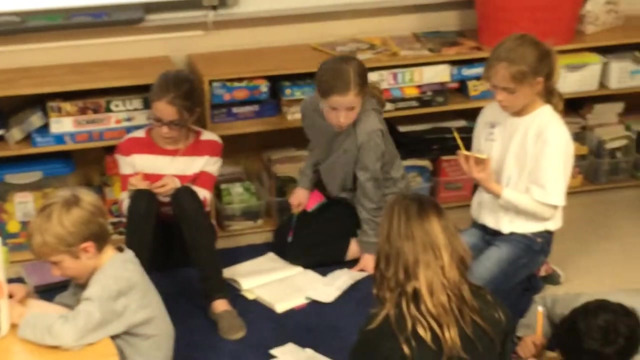 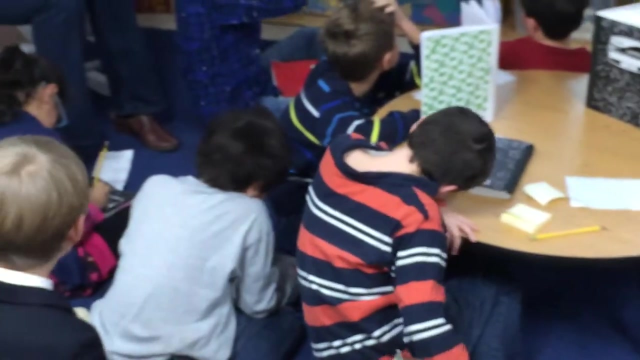 You can start out with. I notice something You can look at: the setting, the people, what they're wearing, what their faces are doing. Yesterday I looked this up on a website and I have probably 15 things in this picture that I didn't notice. 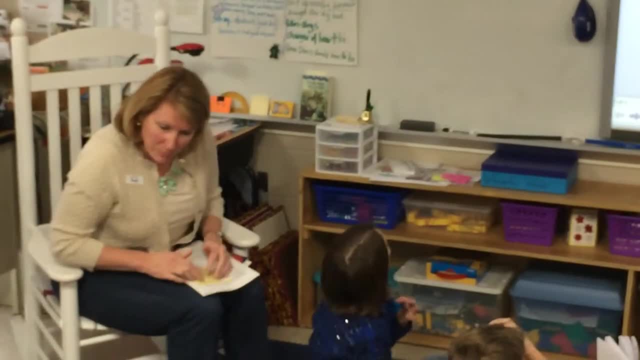 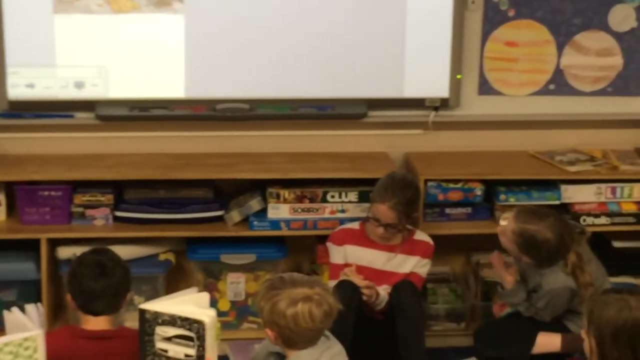 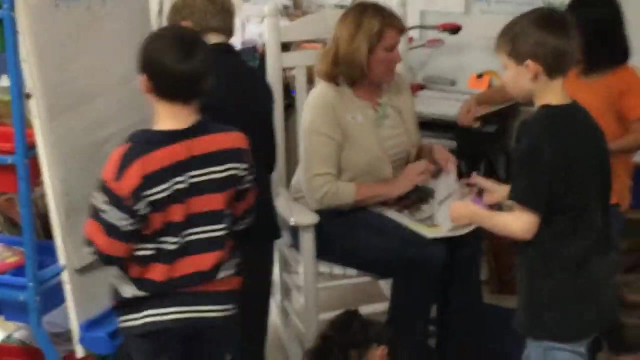 I suppose I looked at it really closely like this and kind of took it apart. Oh interesting, When you're ready and you have some thoughts about this picture, come pop them up here. I want to look at these all together. Is that guns? 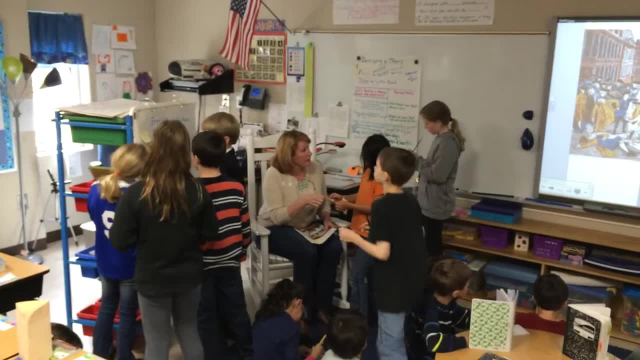 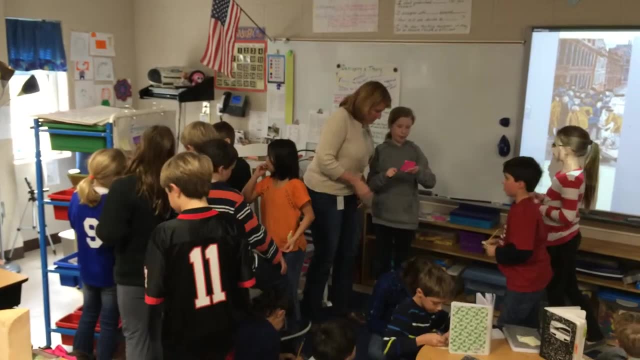 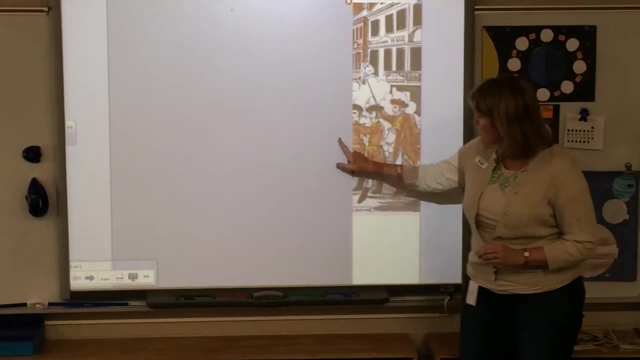 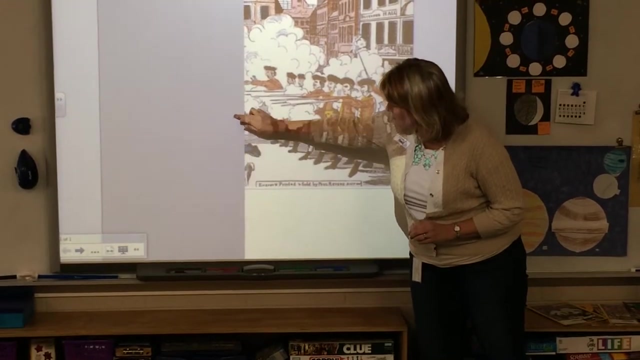 Yeah, Yeah, that's good. Put it up there Ready. Now talk about what you see on this side. Is it the same kind of thing? I knew it, I knew it. You knew it. Yes, Oh, you can see, it's mining. 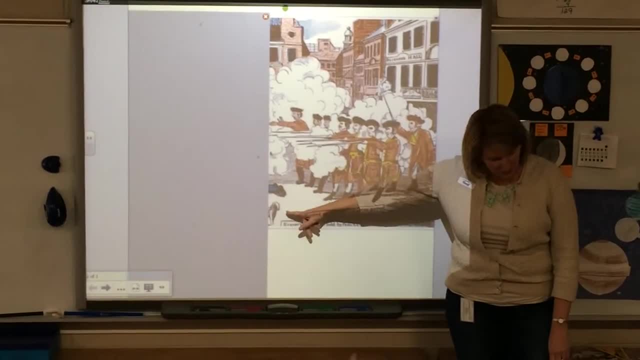 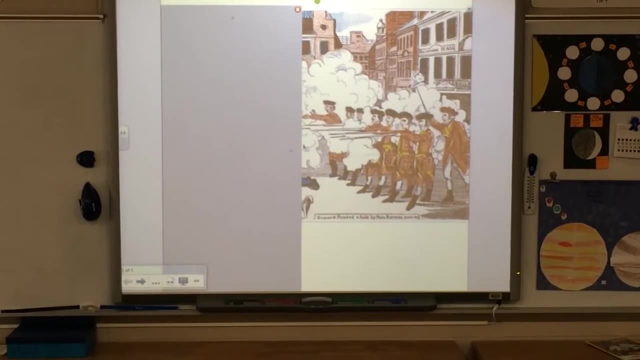 Some oil is mining Well, where There should be more in here, but I wanted that little eye in here. Okay, Oh, wow, Thank you, Ready to? Yeah? Okay, You can even write that as a question if you want. 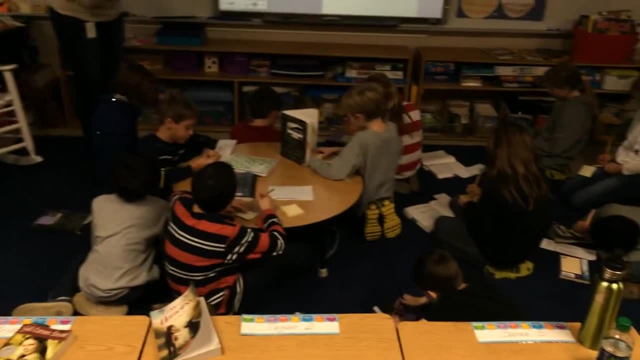 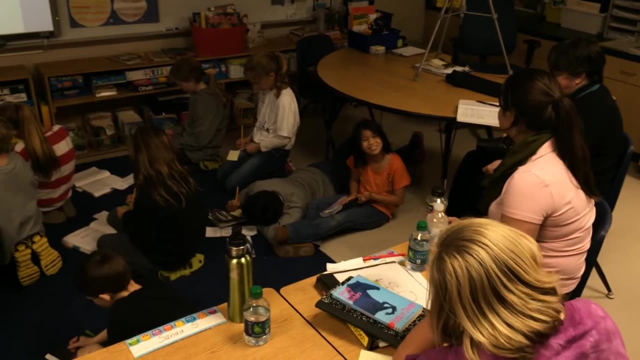 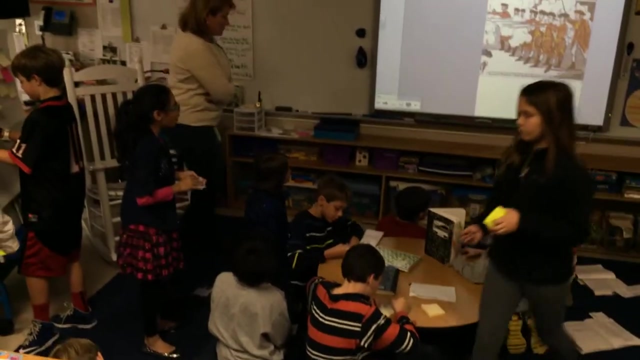 Just like you guys. Hey, I see a dog Write it down. Can we write the legs on there? You can write about anything you notice. If you want to notice that part, I'd love that. That's important. That's a dog. 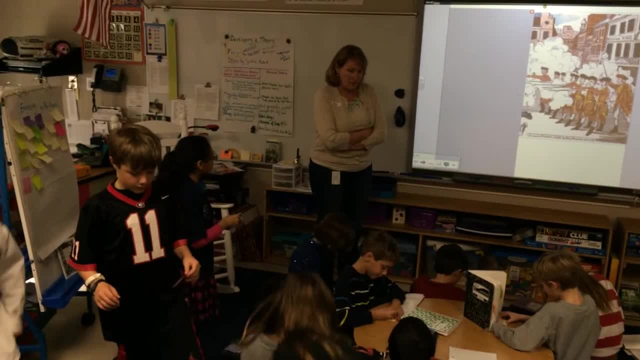 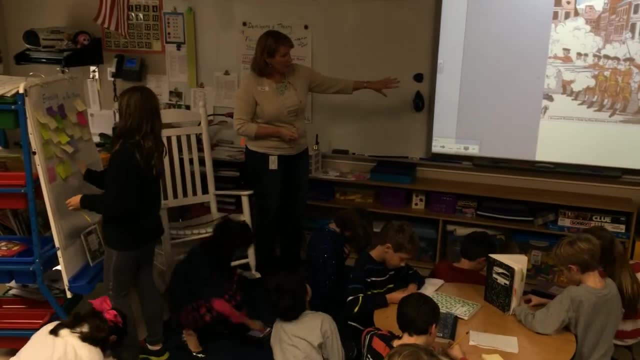 Yeah, write it down. Have you seen the muskets? Just spell it out the best way you can Remember when you write. everything you write is intentional. You have a purpose for everything. Same with this, Everything that's in here. every little line and color and detail has a purpose. 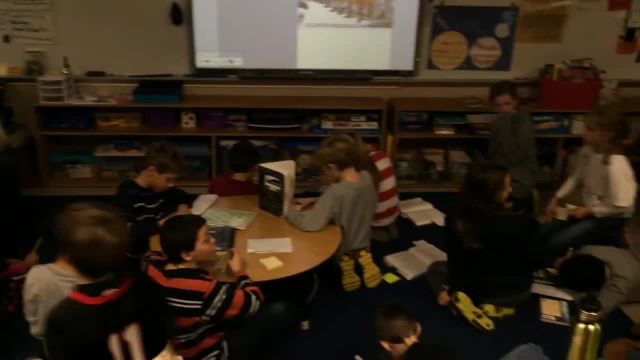 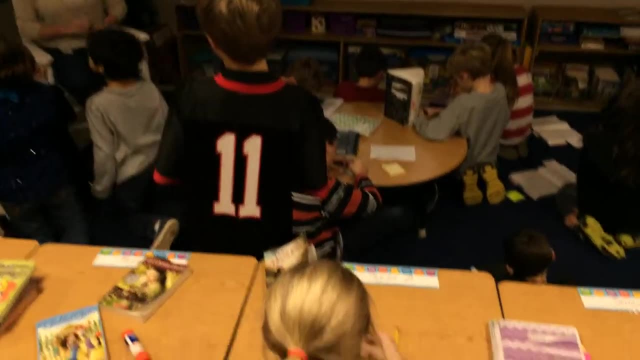 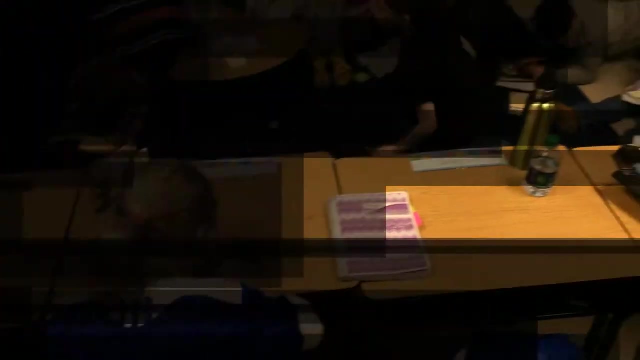 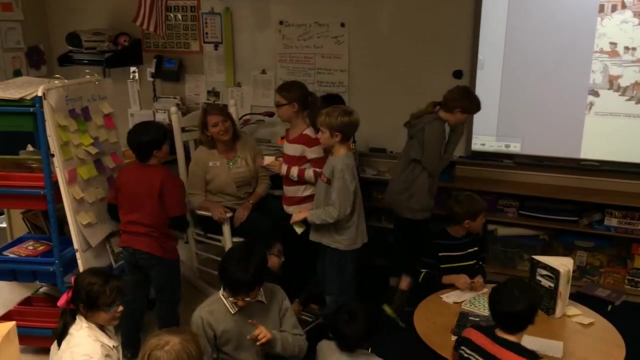 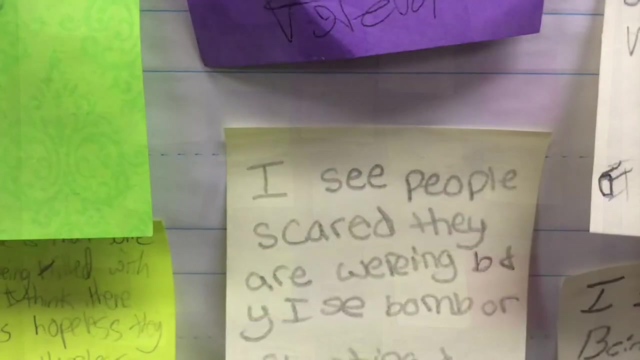 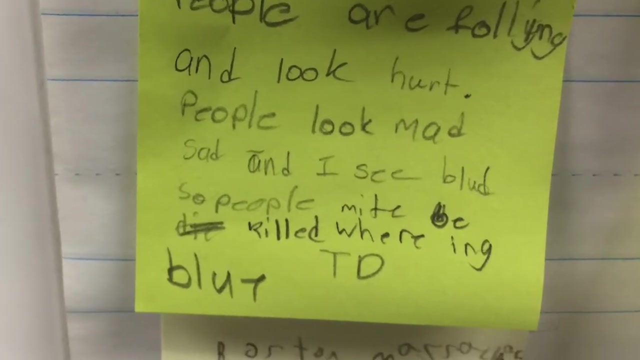 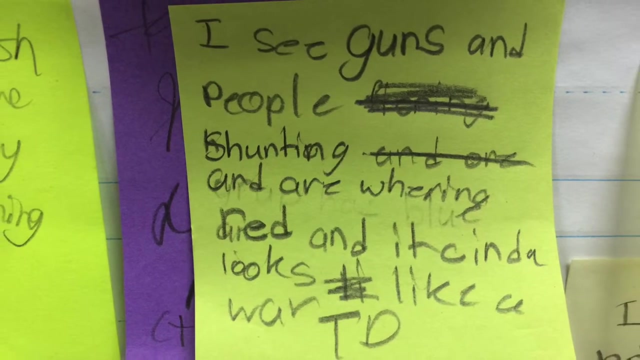 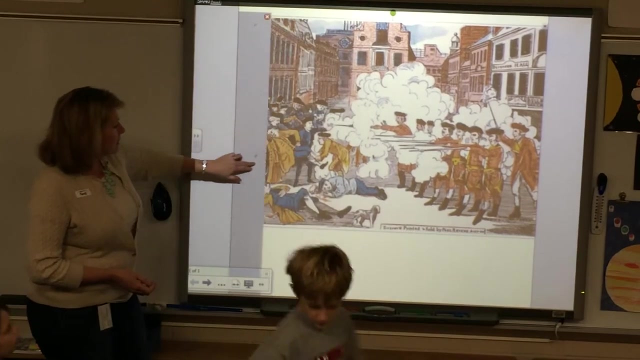 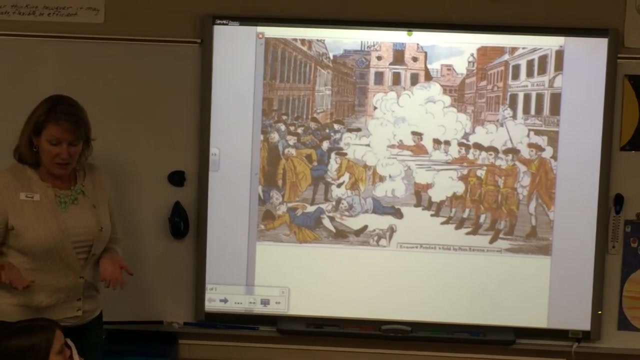 It's intended for you to notice. Can you show this? Okay, Alright, you know what? Let's look at the whole picture. So now we can do this again and put sticky notes on another part of the chart, where we 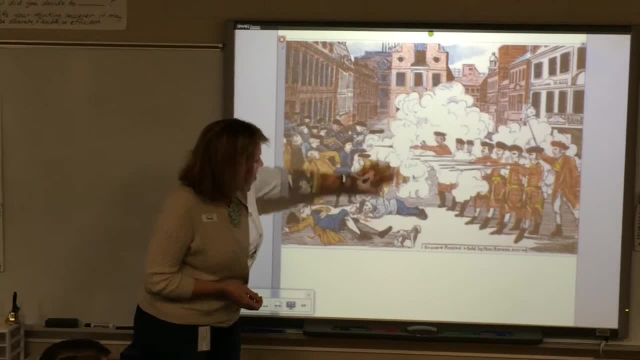 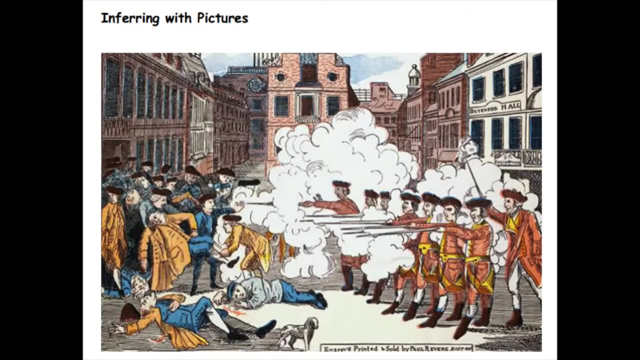 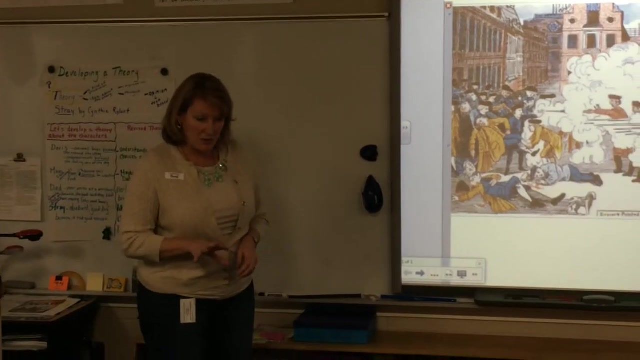 notice. what did we notice now about the whole thing? we didn't even need to see this middle part before. Everybody knows what it is right. What is it called? You can ask her. So I think it's probably better if you get in your table group. 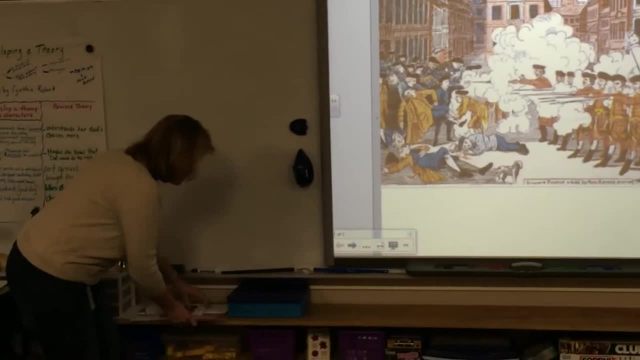 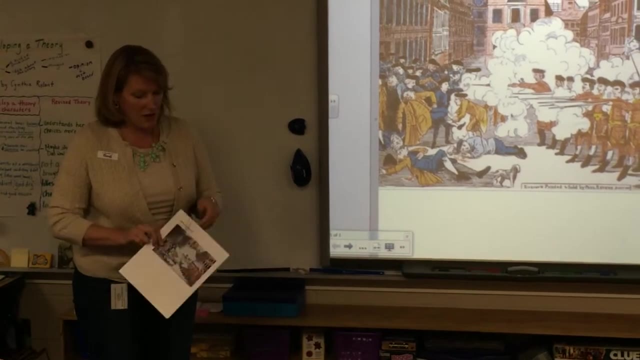 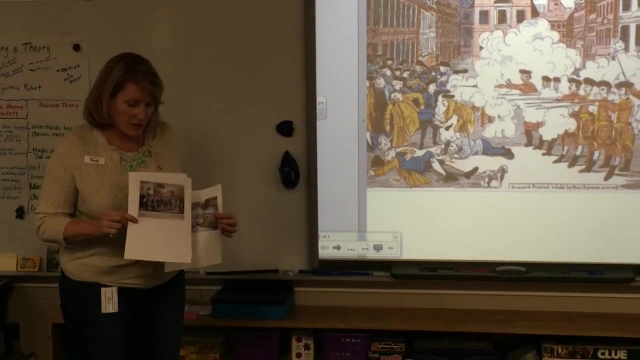 Then if we need to move people around, we will Each, then we'll move people. If three people is good, then you have more time to talk, more chance to talk. So each group is going to get this packet. This picture is in there so you can skip it. we already talked about that one. 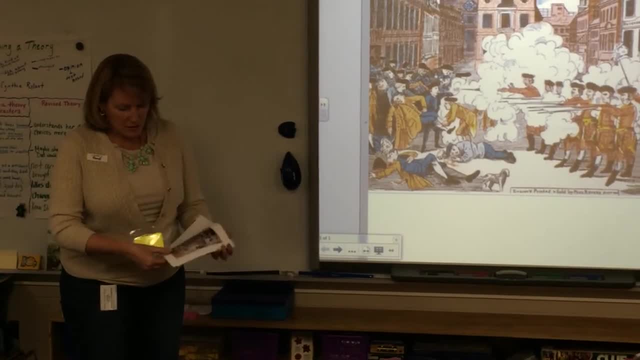 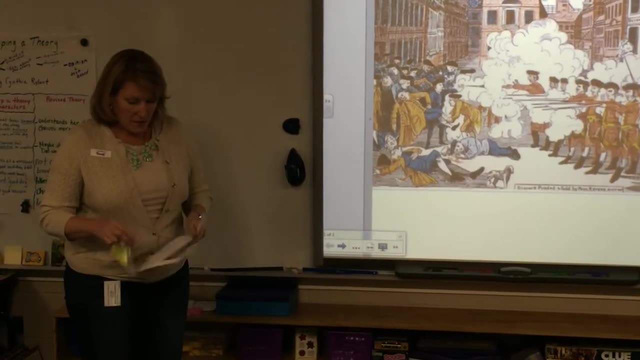 Now you have all of these. some of them are engravings, some of them are drawings. some of them you've seen in your social studies journal already And I've labeled them A, B, C, D, E, F, G, so when we talk about them we can say A- B. 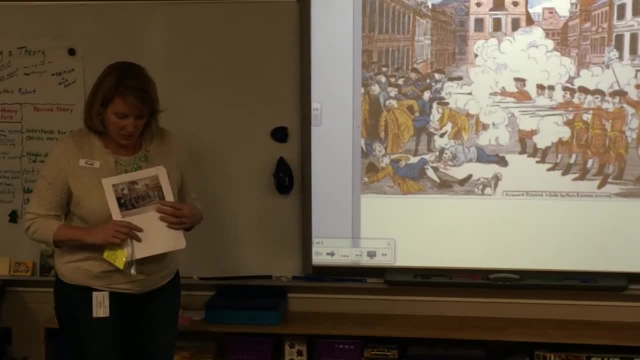 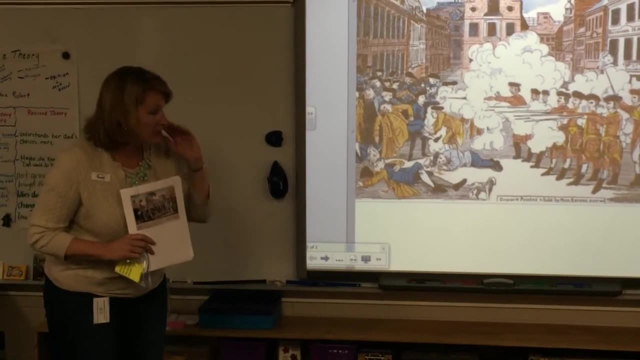 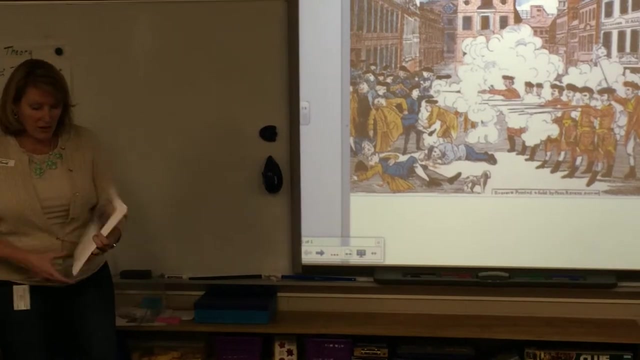 C, this picture- I try not to give you captions or anything like that- And then in your group- I would like it if you did this- all of you stay on the same image, Don't sort them out yet. all of you kind of get around it and look at it together and 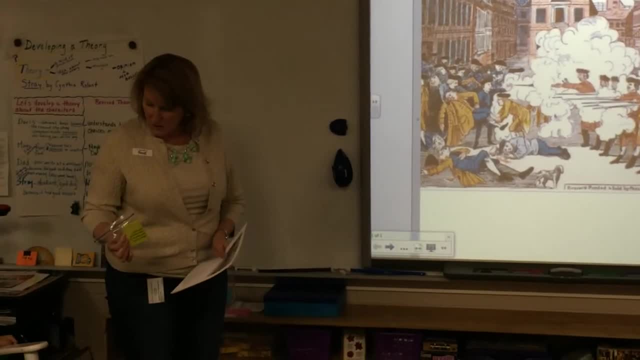 then take some of these cards and ask these questions. pick some of these cards and ask the questions about the pictures, images. Well, why don't you go to your table groups and then we'll move people around. So go back to your table groups, take all of your things. 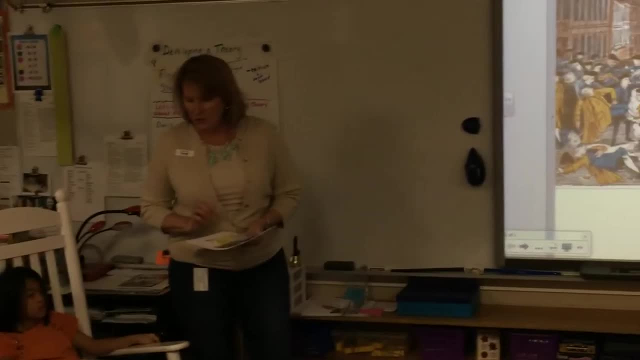 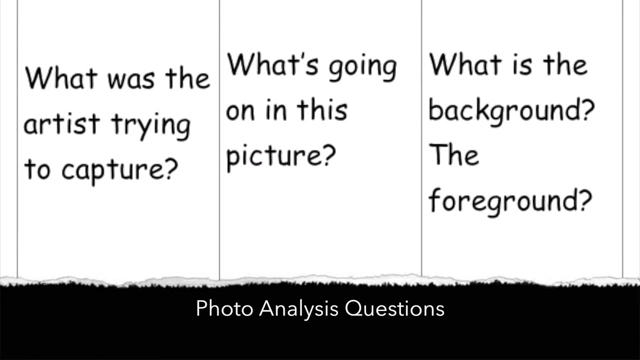 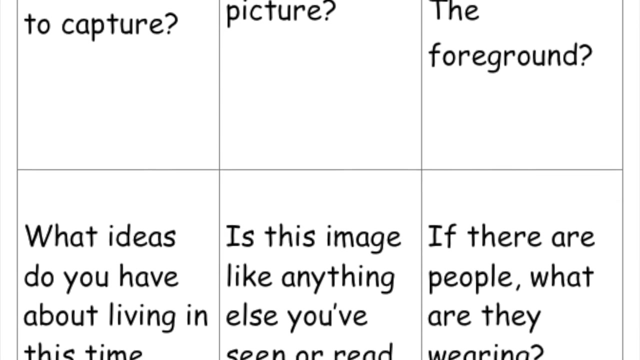 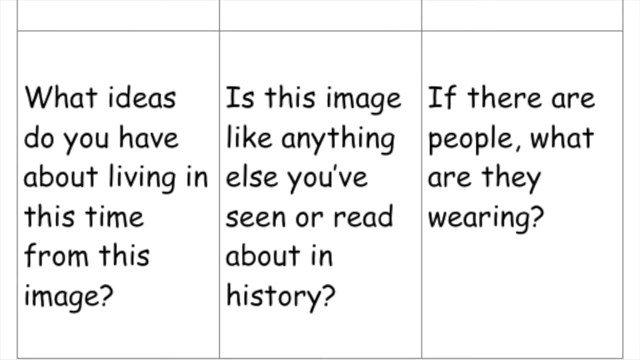 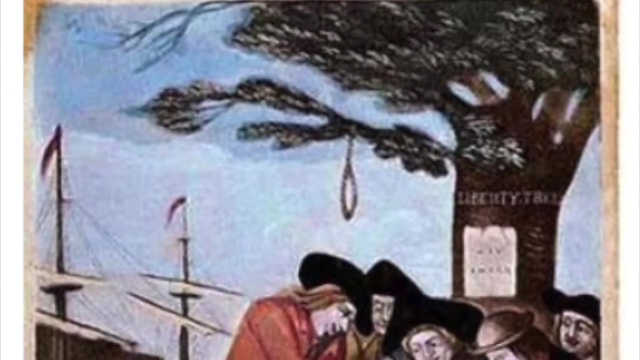 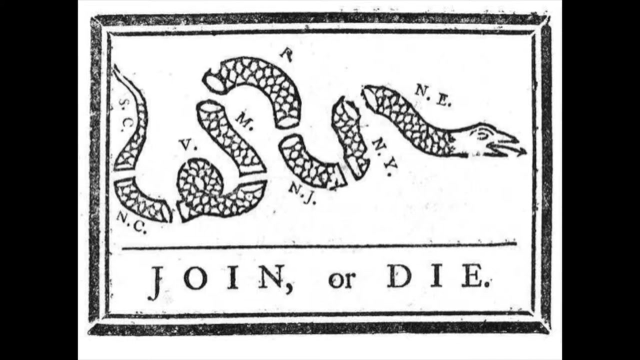 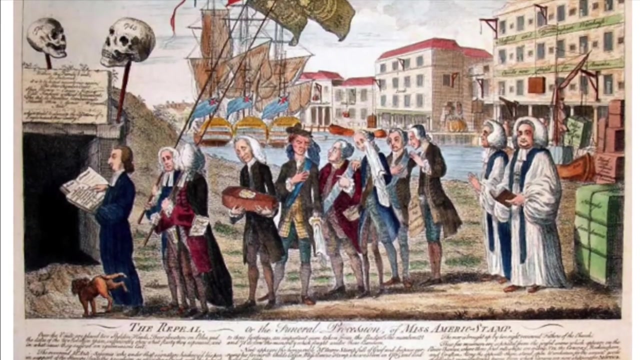 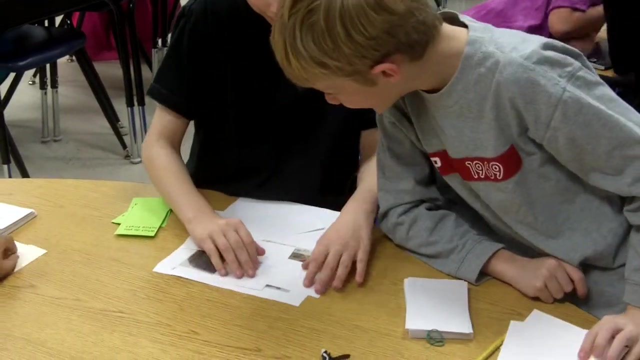 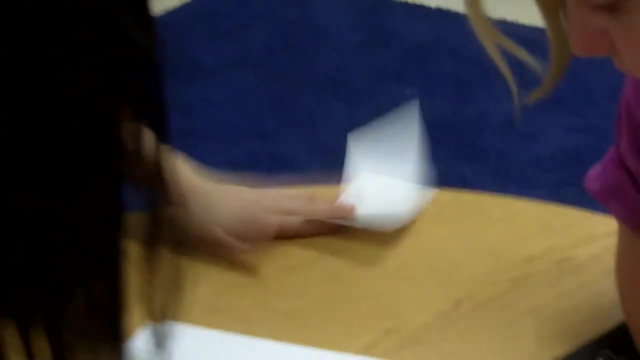 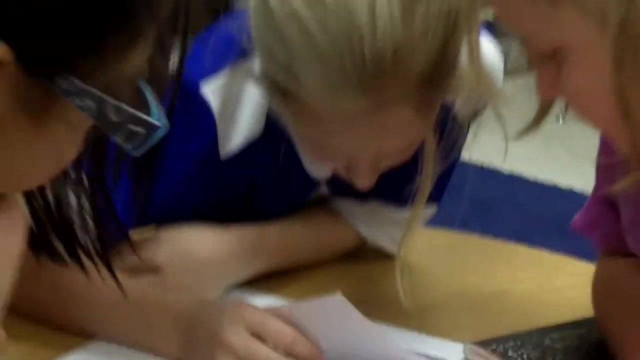 I can't see that. I can see it right here, Simon. Wait, what do these words say? It says like D: Okay, I get it Um one. I can't see it, Guys. I guess what this says is that the 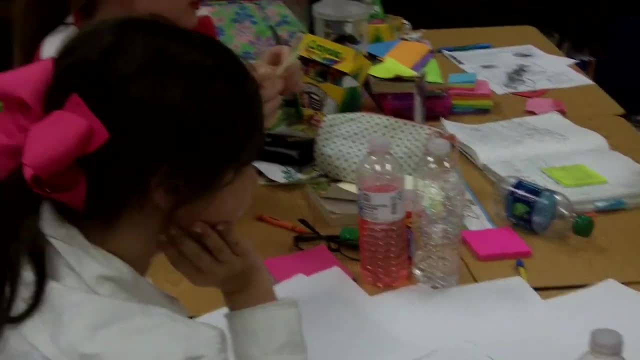 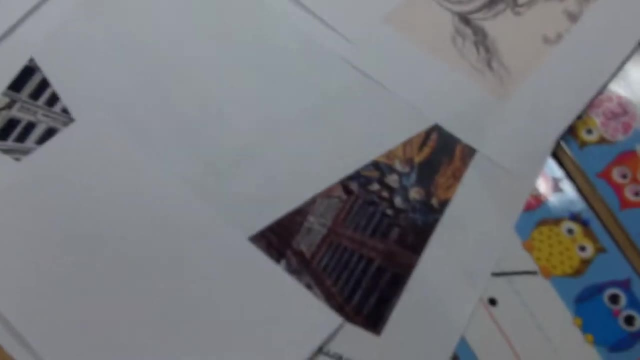 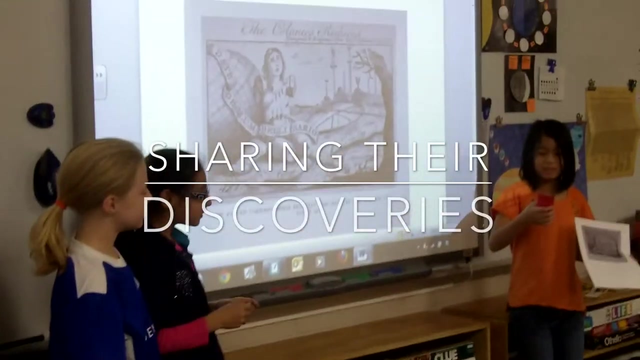 car is reduced. Okay, What do you notice first? What do you notice? The tail. What is that? Is someone riding the horse? as you can tell, It's the little saddle. This image is like anything else you've seen or read about in this. 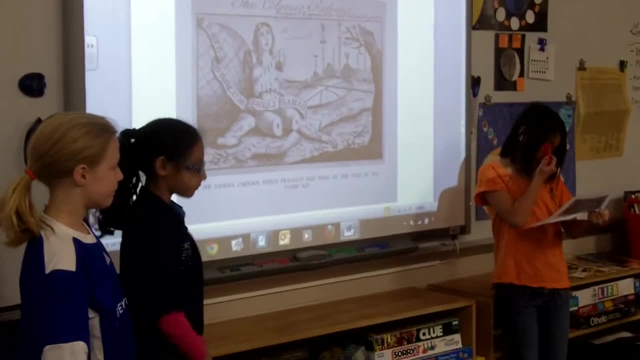 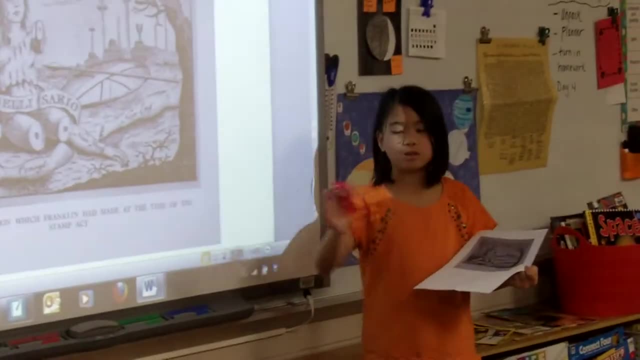 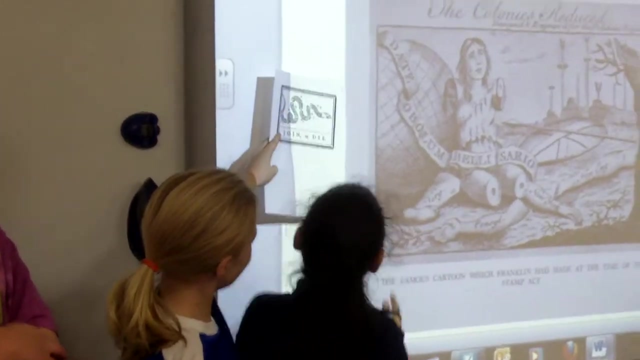 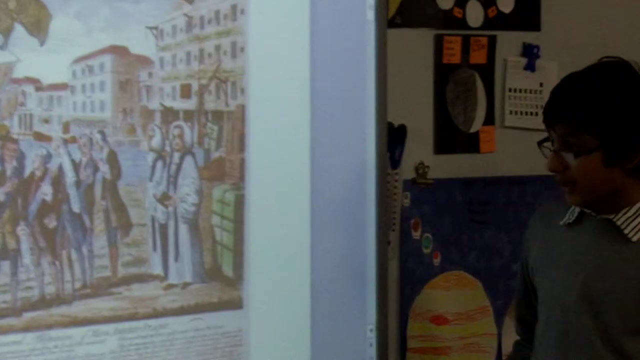 in history And like this one shows about all the countries separating stuff And that snake one kind of like this one, because like all the plants are all separated and they look like that. He made a cartoon that went away. He made it like a cartoon. 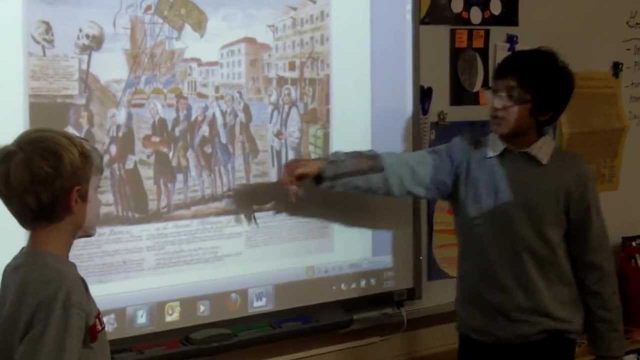 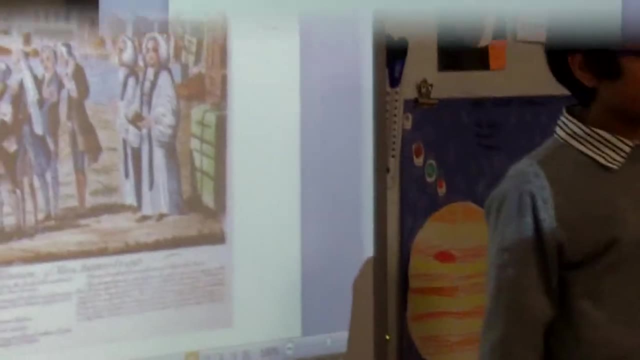 Like trying to make it like funny, That they made like all There's these guys and stuff and all these people are sad, Um, and the stand backs look like. Uh, I noticed that the guy was holding like